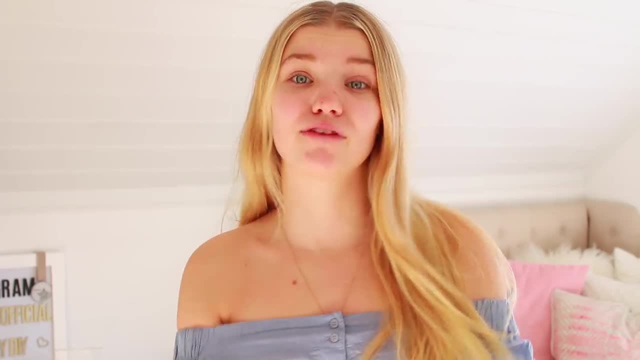 I've, like, updated everything. I'm super excited to hear you guys, So if you want to prove to everyone on YouTube that the mace relay squad is the best squad to be a part of, then make sure to click the like button and let's get this video to. 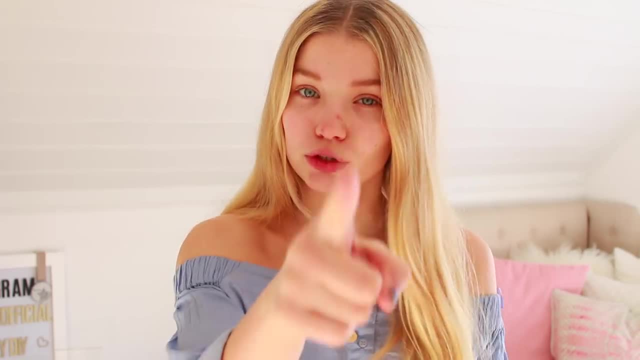 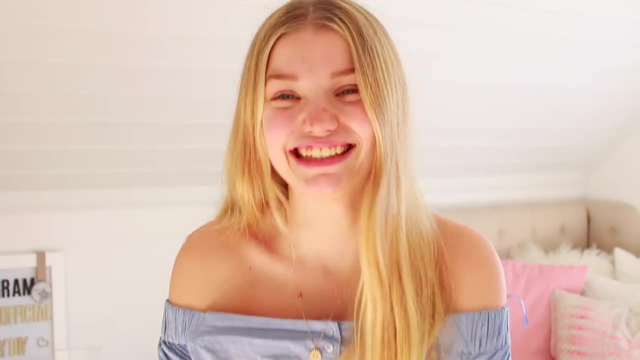 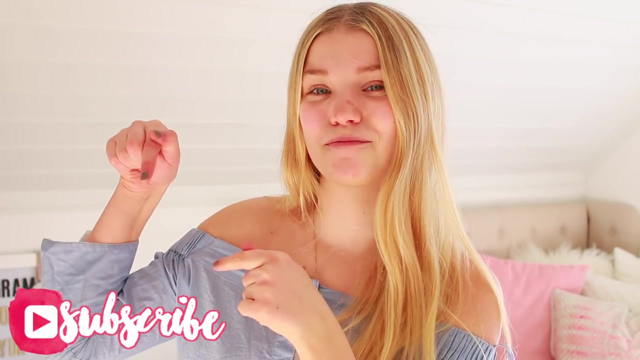 15,000 thumbs up. Is that possible? So you right there, don't debate on it, Just click the like button. I'm waiting for you. Oh, If you're in a part of the mace relay squad already, Which is the coolest squad to be a part of on YouTube, then make sure to click the subscribe button and put on post notifications. 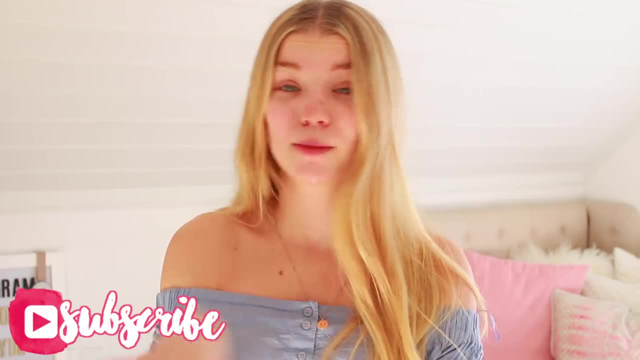 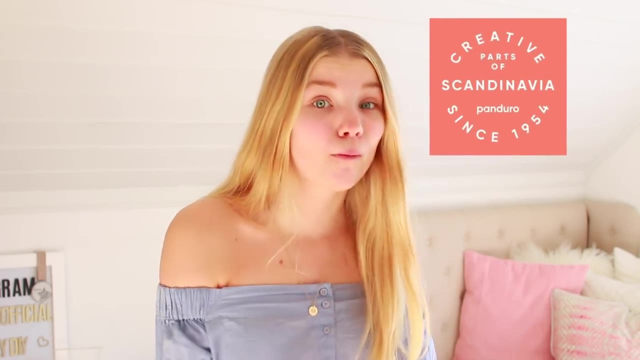 Because it's spring and the videos are just coming on a roll. Is that even possible to say? I don't know. So obviously this video is a collaboration with Pandurahobby, Which is where I get all my craft supplies for this video and all the DIY videos that I do. 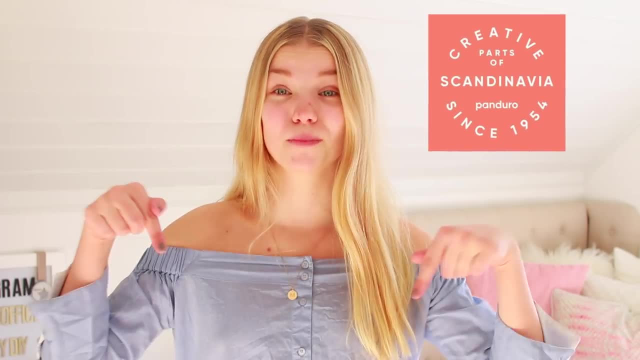 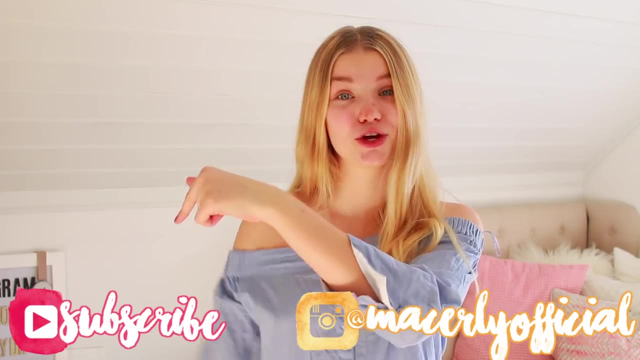 They also sell a lot of organizational stuff- You should definitely check out their website, which I will link down below- and they also have stores in Norway, Sweden and Denmark. So yeah, I think that's all. Follow me on YouTube. follow me on Instagram. 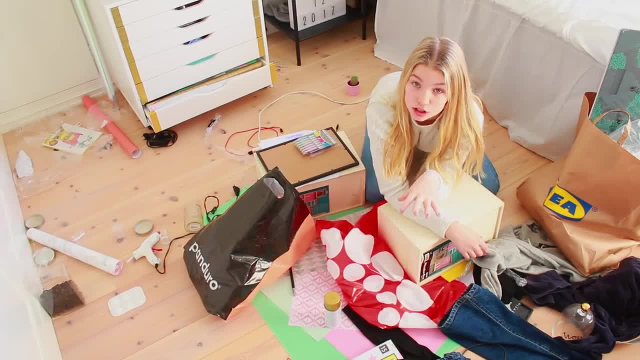 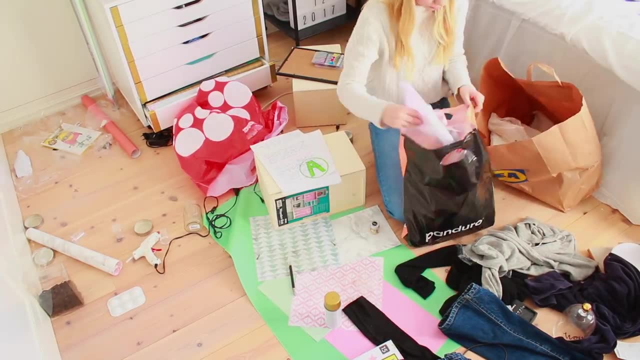 Let's get right into this video. I swear the hardest part of Cleaning is just starting, So Let's do this together. Let's go So. obviously, since my floor was a disaster waiting to happen, The first thing I did was sorting out everything from trash. 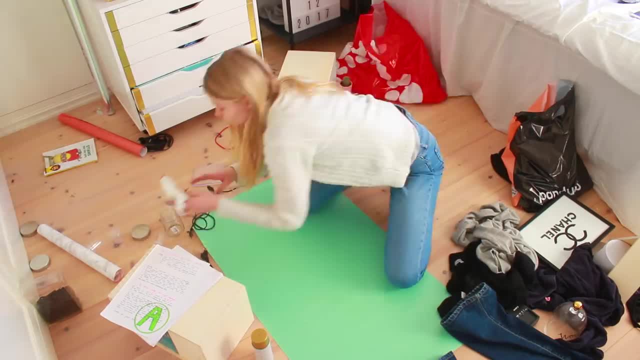 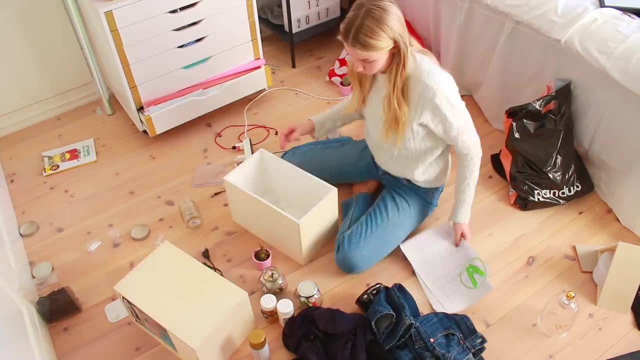 Stuff that belongs somewhere else, stuff that should be organized and clean clothes and dirty clothes- And I'm sure you guys have some deep feels about the chair, the shelf or, in my case It's the corner of my room on the floor, where all my dirty clothes always end up. 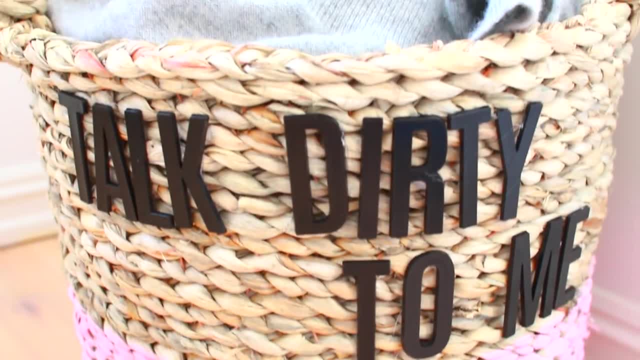 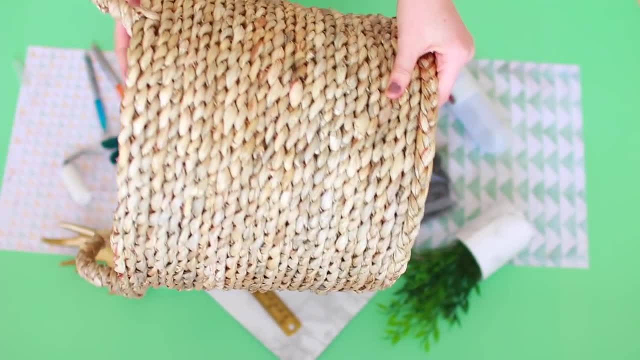 So let's DIY a super cute, yet very useful basket. You'll need acrylic paint, a sponge brush, 3d letters, a glue gun and a decent sized basket. However, it shouldn't be too big, because they'll just end up never emptying it, which is not what we want. 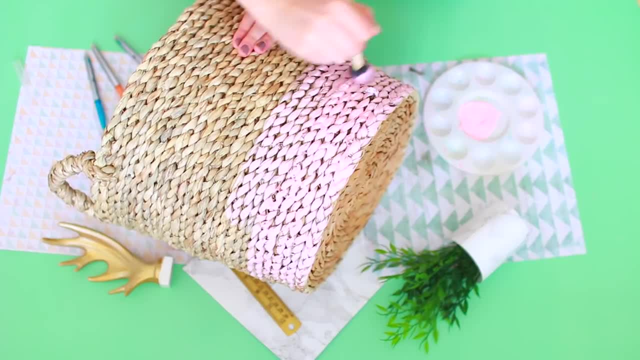 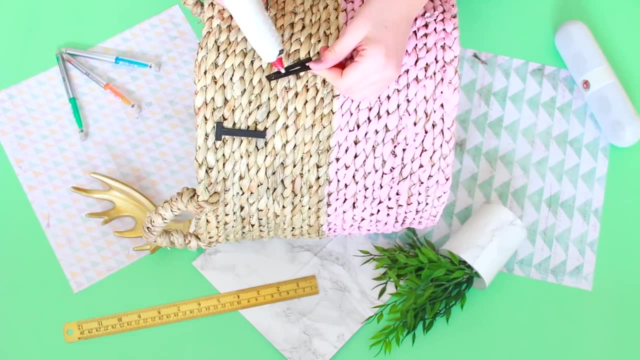 Anyway, the first thing you want to do is dab on acrylic paint to the bottom half of the basket, Wait for that to dry and grab your glue gun. Now I decided a funny quote or saying to spell out with letters Which I hot glued onto the basket. but you can spot anything from your name to a cheesy quote, like with a: 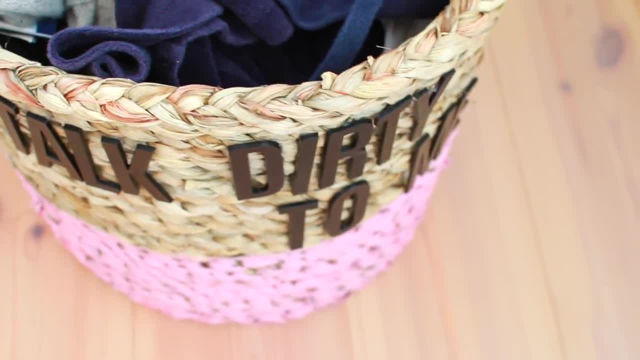 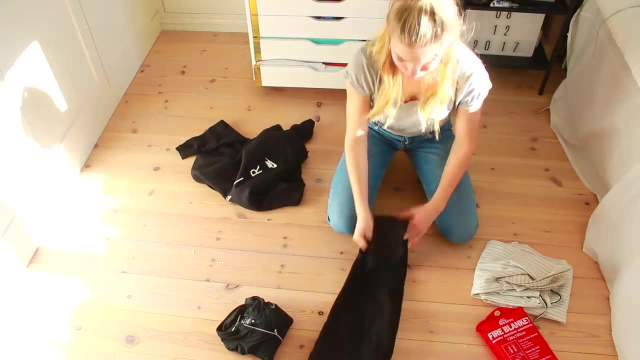 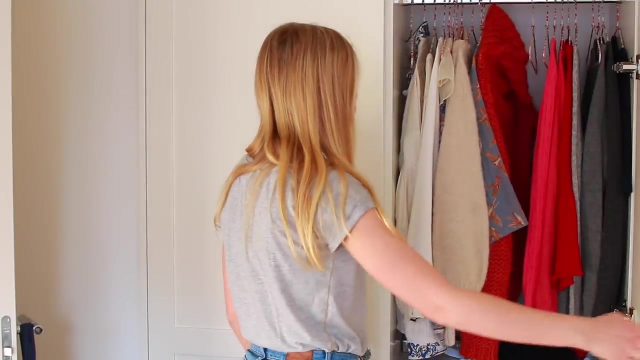 Great power comes great electricity bills, or probably not that, but you do you All right. so, with all the clean clothes, I either fold them and put them back into my drawers or hang them up in my closet. However, I've been using these hangers for like three years and, even though they're cute and stylish, Sometimes it's nice with a change. 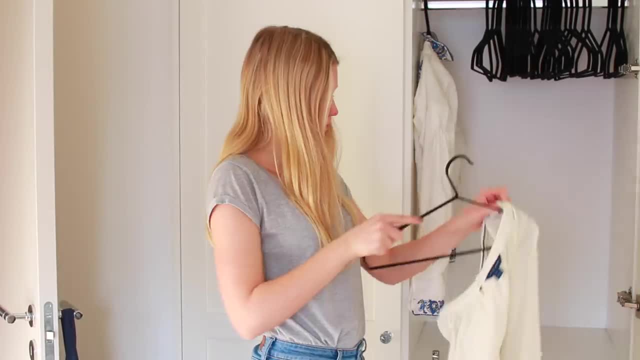 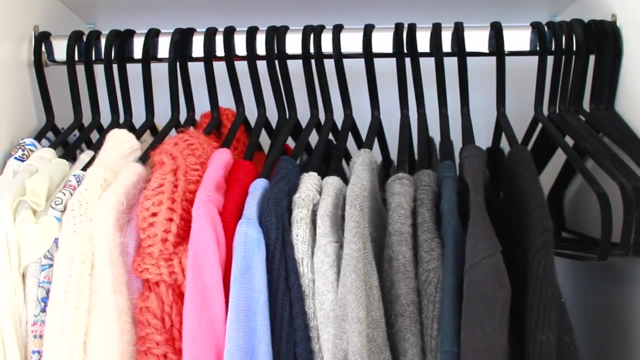 So I got these velvet clothes hangers from Ikea Scandinavia represent. and they're great because the velvet clothes hangers from Ikea Scandinavia represent. and they're great because the velvet clothes hangers from Ikea Scandinavia represent. material stops your clothing from slipping off the hanger, which is super annoying, but you guys look how clean and neat this looks amazing. 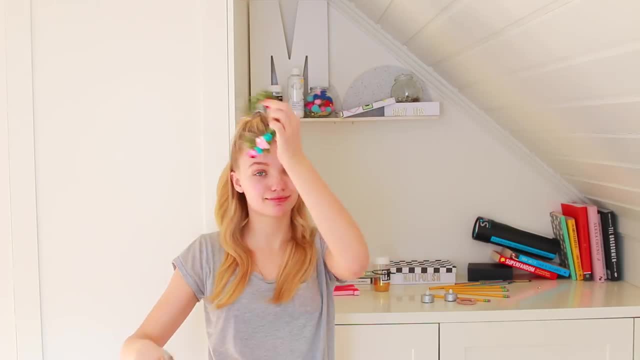 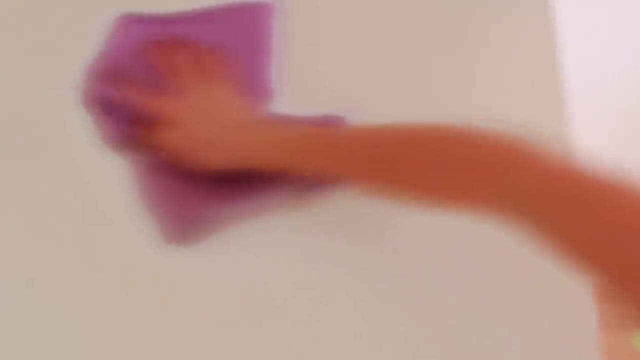 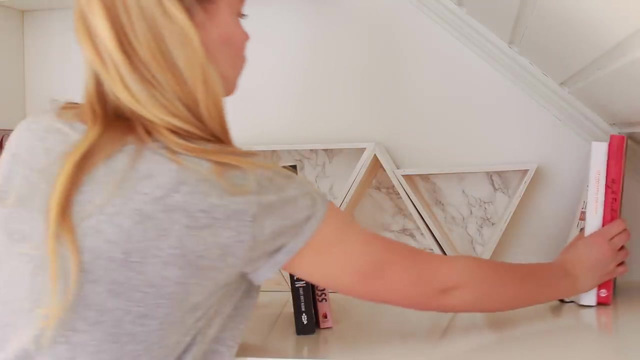 Moving on to the top of the dresser, which is the area I believe has the most potential in every room. So let's make it beautiful. Starting off, I removed everything and cleaned the surface, because it was really dusty, and Then I placed in these five triangle boxes from pandora, hoppy, and I used them both as book stand, on either side as well. 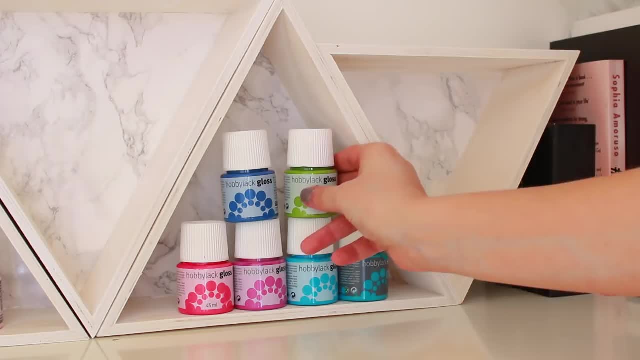 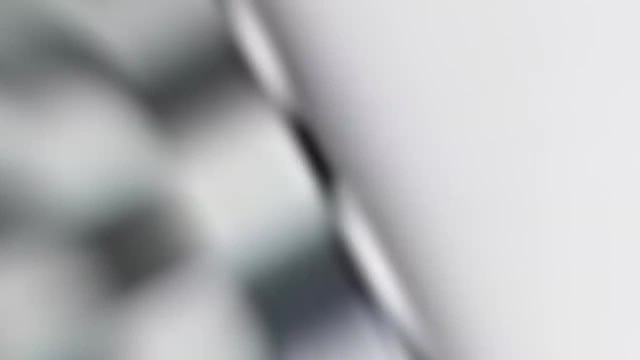 As a place to store my new duct tape. So I'm going to use these duct tapes from pandora and acrylic paint. Want to recreate them. you'll need triangle boxes, white paint, a paintbrush, marble, contact paper and an exacto knife or a pair of scissors. 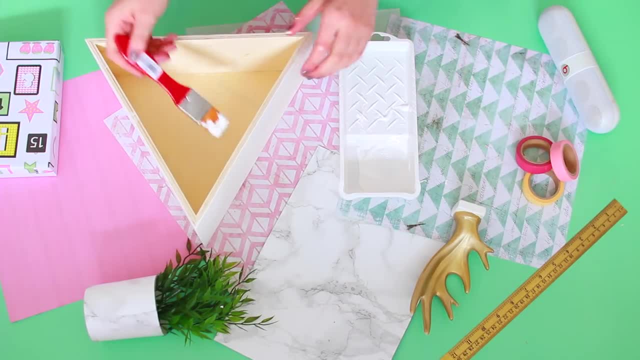 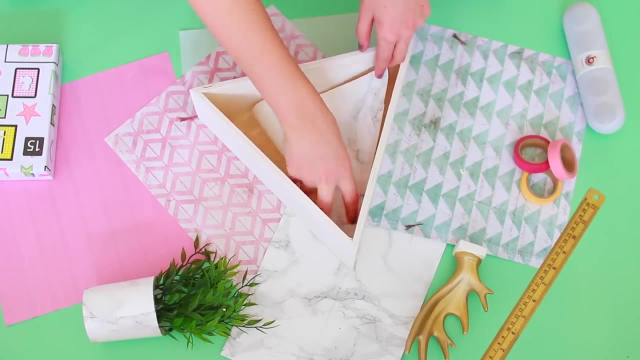 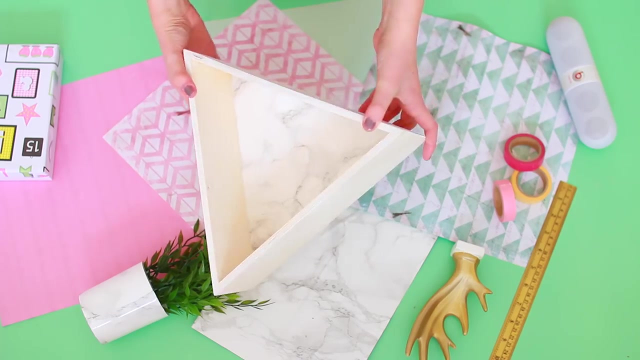 Firstly, go ahead and paint both the inside and the outside of the box with white, Cut out the contact plastics to fit the inside of your triangle, peel off the backing and stick it right onto the inside, And if you get any air bubbles, Simply use a flat object to smooth them out and viola easy right. 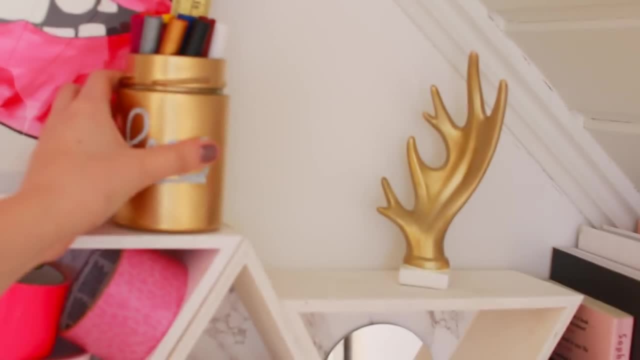 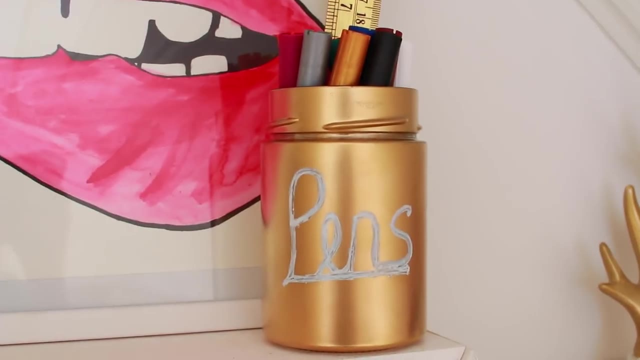 To decorate this area a little bit. I framed my water color painting and I added this amazing gold pen holder as well as it's mini gold organizer. and guess what? They're both DIYs too. to make them yourself, You'll need a stamping block, a glass jar in mini cylinder boxes or mini glass jars. 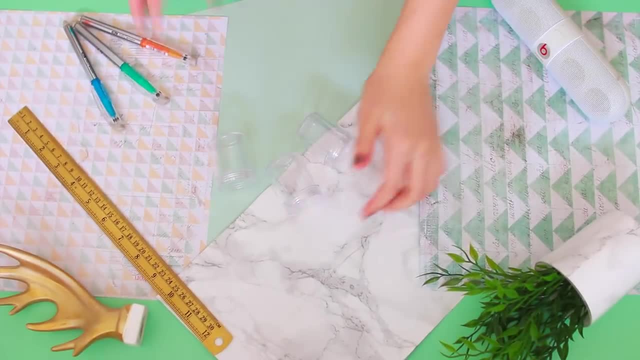 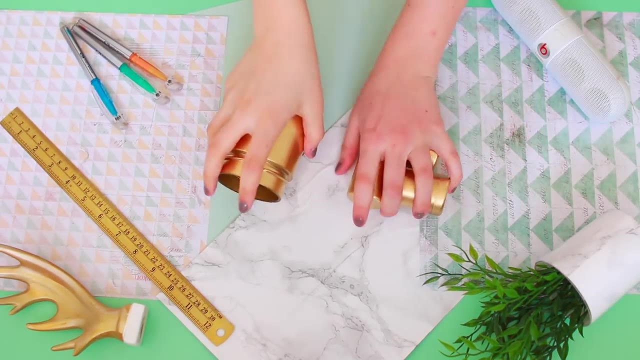 gold spray paint, pictureойдles and evaluation paper paint, a glue gun, glass and porcelain pens and a marble contact plastic. First off, spray paint all of your jars gold. cut out the contact plastic, a little larger than the glass stamping block, peel off the back and attach it right onto the block. 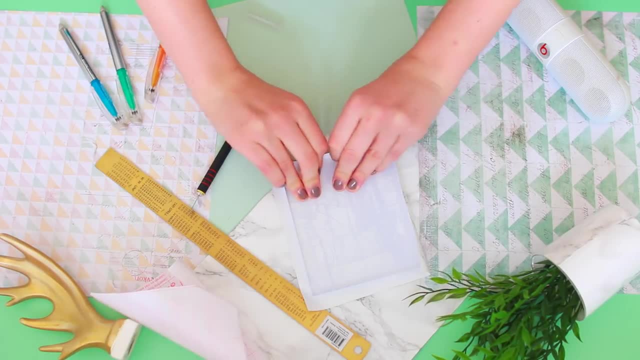 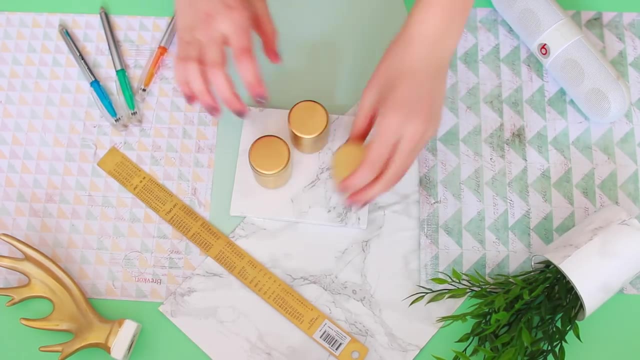 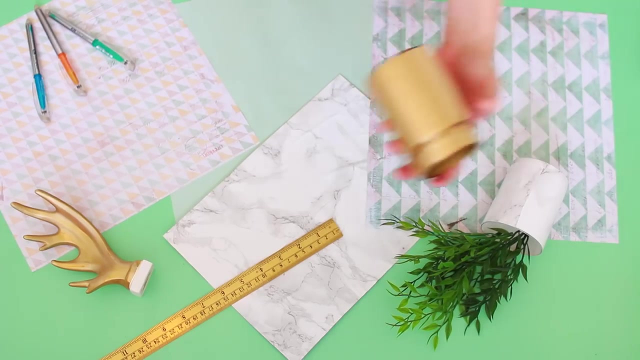 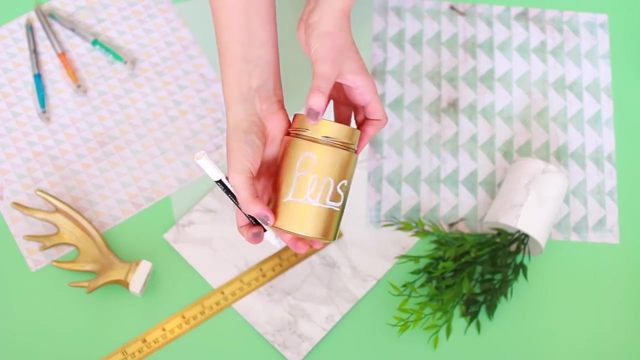 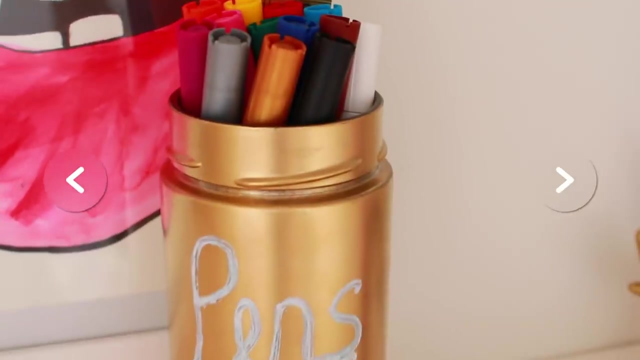 And if there's any excess plastic, simply run your knife along the edge to remove it. Afterwards, hot glue all the mini jars to the block and on the bigger jar, write on whatever you want to put inside with your porcelain pen. And I chose white because I think it looks pretty cute. 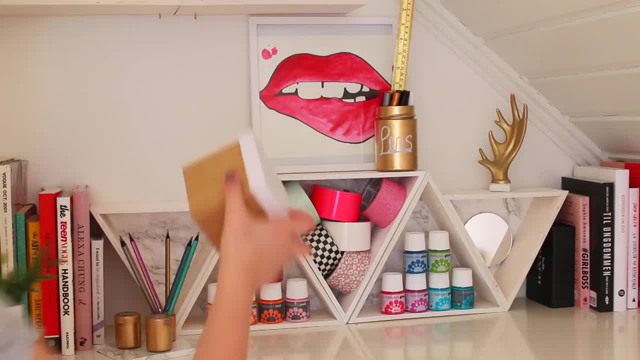 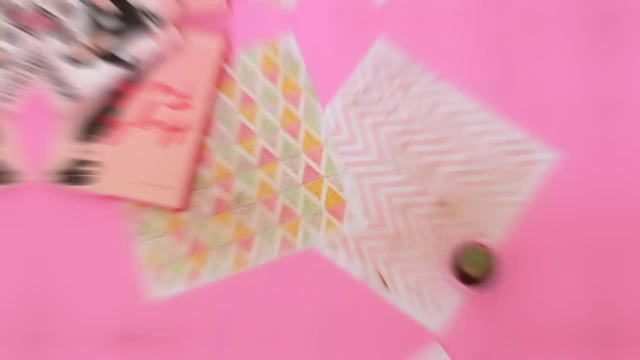 And there you have it: Super cute organizers for all the smaller things in your room. But what about those bigger, harder to organize items? To make this box you'll need White boxes, acrylic paint, wood, contact plastic, an exacto knife, a flat object and a paintbrush. 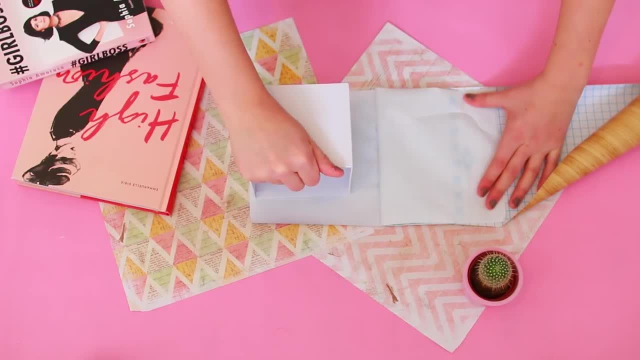 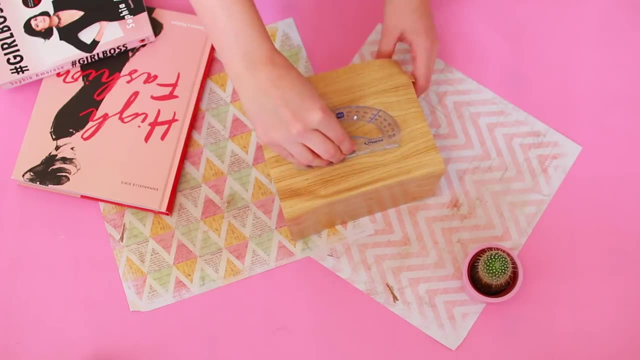 Go ahead and put the lid aside and attach the contact plastic to the box as so. I find this rolling mechanism to be the easiest way to avoid air bubbles. Grab your exacto knife and, like wrapping a book, cut every corner and fold the sides. 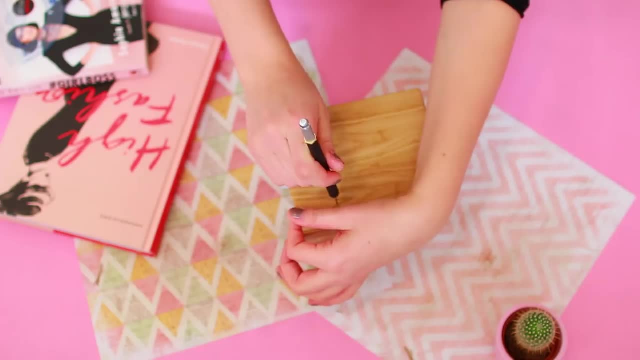 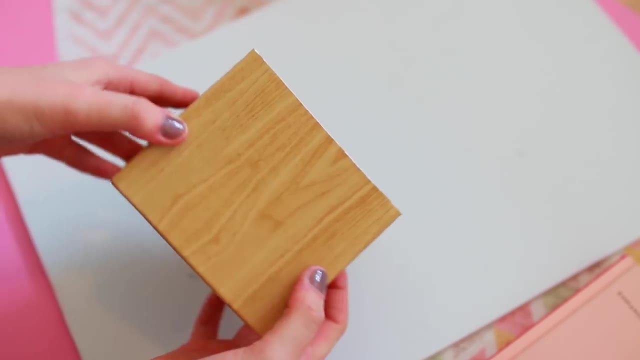 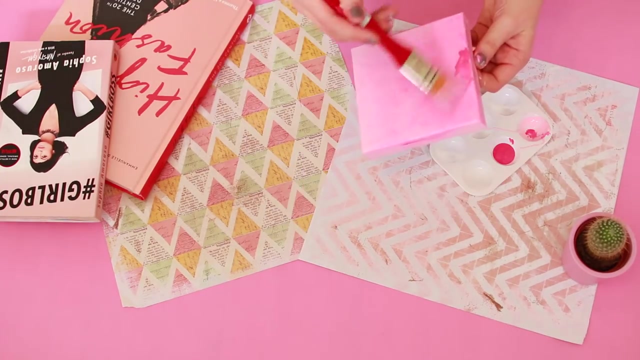 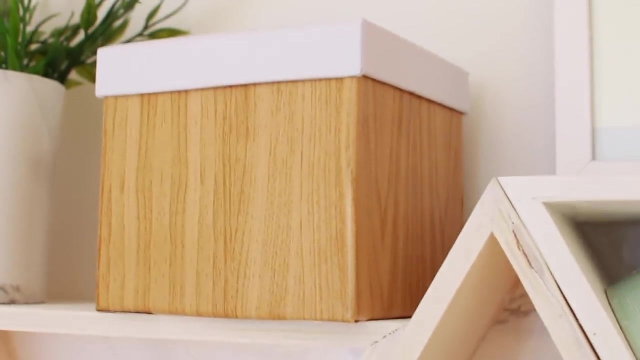 in. Flip the box around and, as we do with the marble block, slide your knife along the edge to remove any excess. Last but not least, paint your lid in the color of your desire, or just leave it as it is. I filled up one of my boxes with glitter, and, even though glitter could be pretty on. 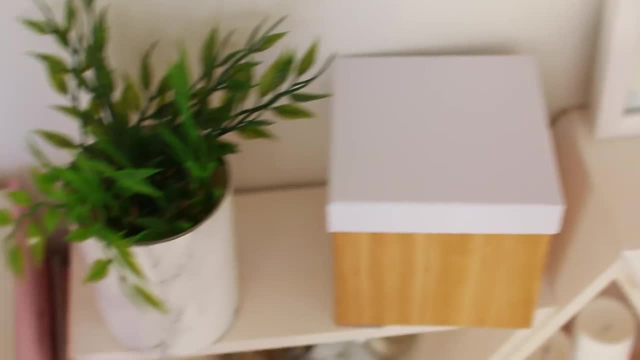 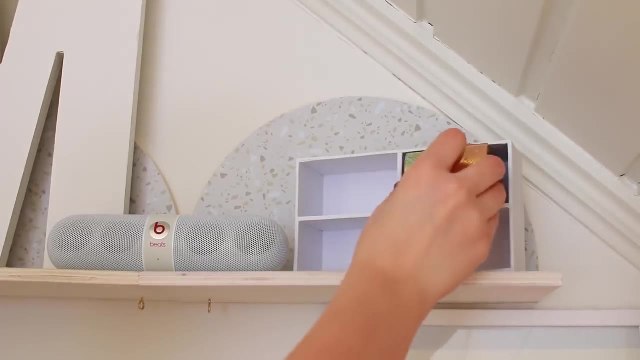 its own. storing it in this box makes Manchester's surface look much more organized. To finish off this area, I added a bead speaker and a small organizer. I've got this from my store and I'm going to be using this as my dressing table. 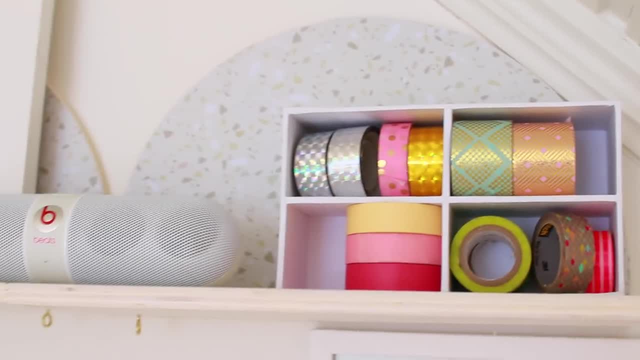 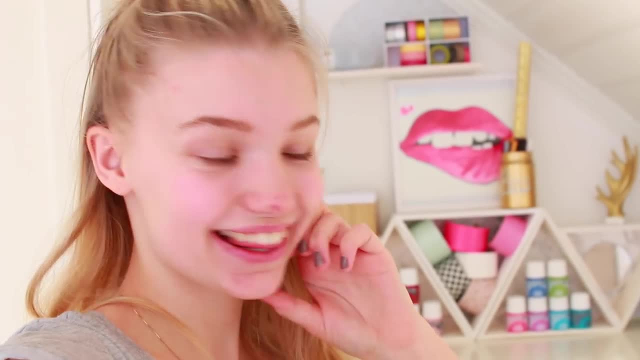 I'm using this as my dresser And guys, I'm not going to lie, I'm kind of in love with this area right now. It's nice, I like it. I promise to be there in every single way. We're doing this together. 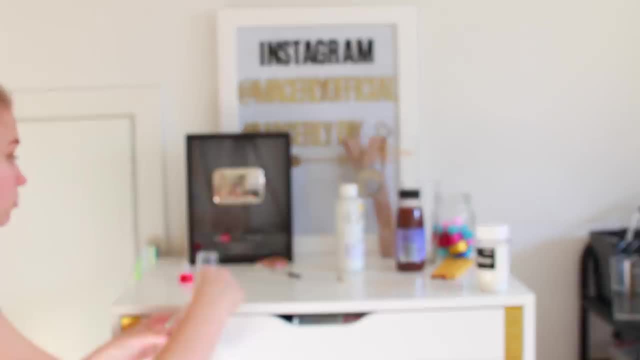 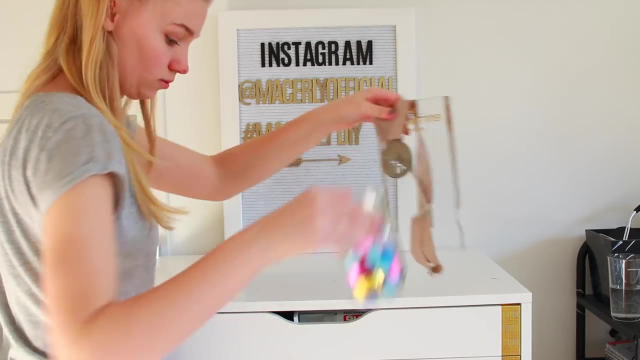 That was not close. Oh my gosh, Oh that Alex drawer. Why did my surface become so unkempt As I did with my dresser surface? I removed everything and cleaned off the surface that was not closed. oh my gosh, oh thy Alex drawer, why thy surface become so unkempt as I did with 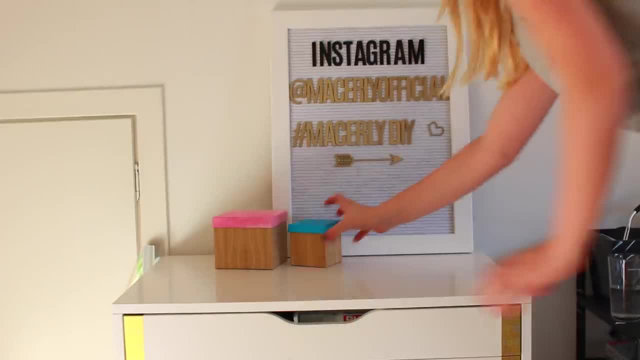 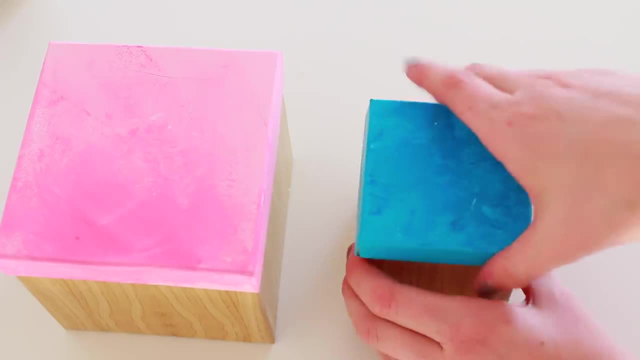 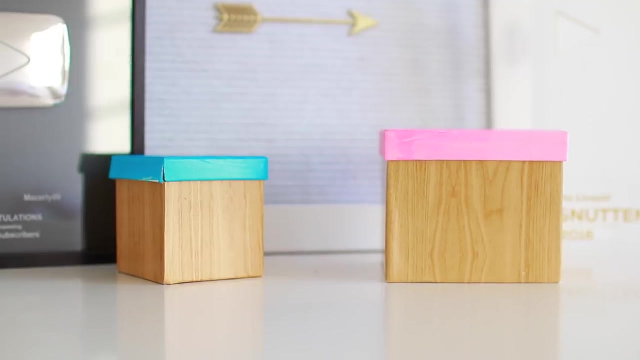 my dresser surface. I removed everything and cleaned off the surface. however, this time I placed on two of these organizational boxes which I filled up with baby lips and nail polishes. luckily for me, the drawers are still decently organized, so cleaning this was pretty simple. however, if you want to know how to declutter your drawers, I will leave a link to my video. 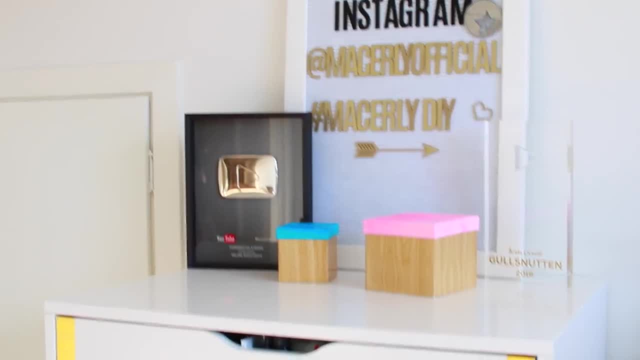 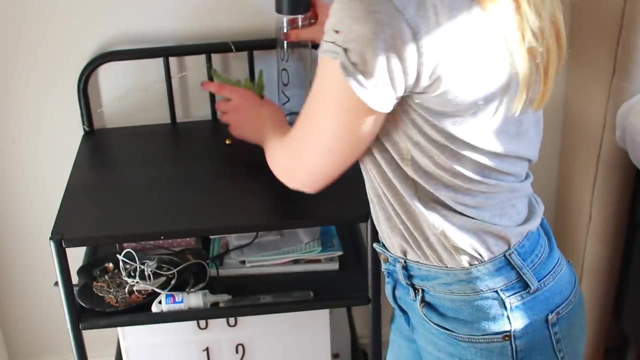 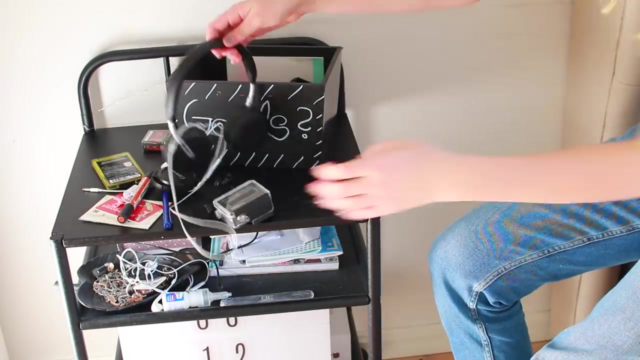 about that topic in the info box. night table nightmare in my case. yes, first off, to clean my night table, I remove any trash or used up water bottles or nasal sprays. hey, don't blame me for the awful flu season. though for the other must-have items, I placed them into this organizer. 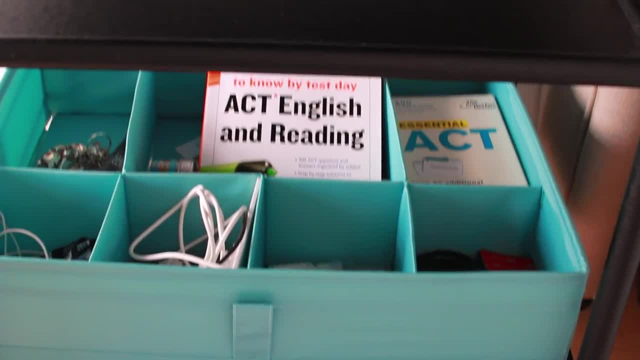 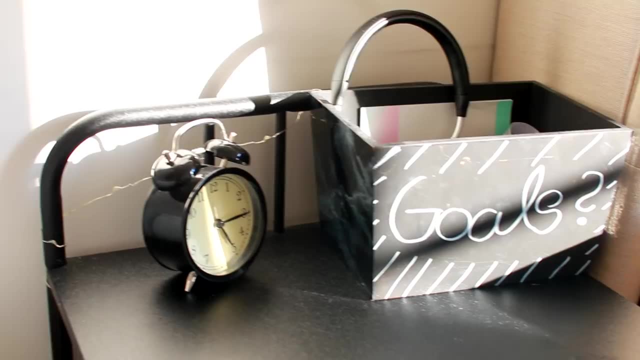 from Ikea, which is supposed to be for your drawers, but hey, it worked great here as well. lastly, I put back some of my books. the spin my clock and baboom nightmare to daydream in less than five minutes, thank me. later now let's tackle the bed. 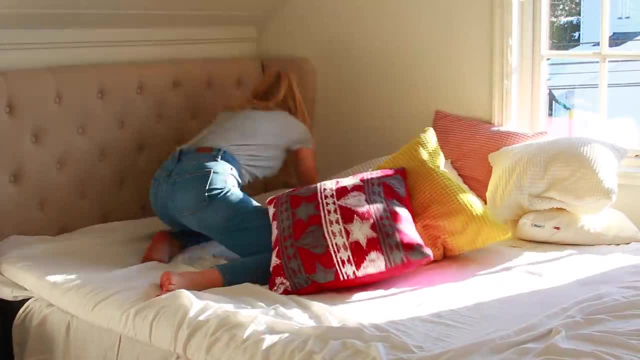 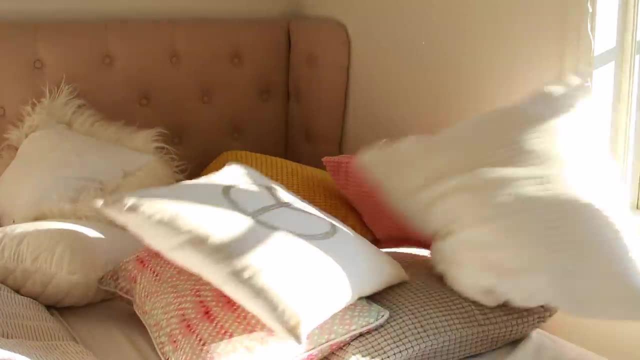 area which, in all honesty, I wish I had a hack or DIY for to make it easier, but sadly there is none. you just have to make your bed to make it look nice. I really don't like making my bed. it takes a lot of time, but it's all worth it in the end. 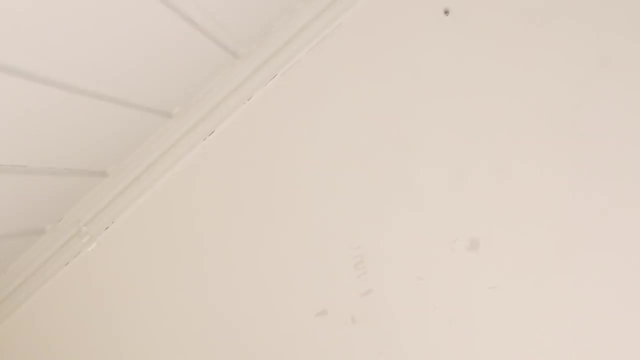 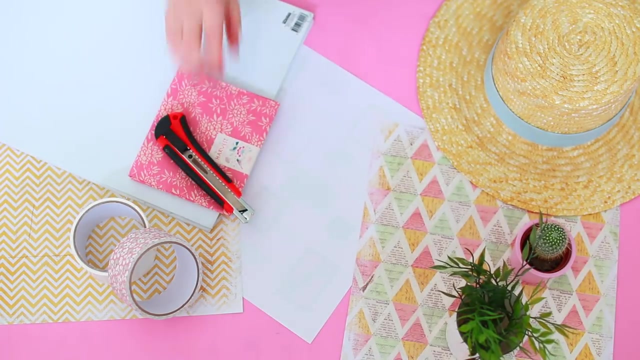 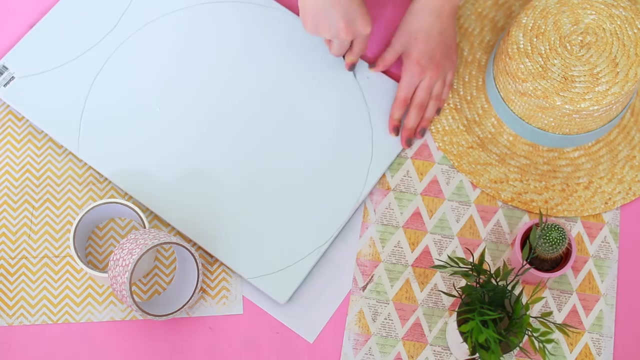 on the other hand, I do have a DIY for this boring wall. to make this pink pin board, you'll need a foam board fabric, a craft knife, an exact knife, a glue gun and yarn or thread. to begin with, you're going to have to make two identical circles which are smaller than the 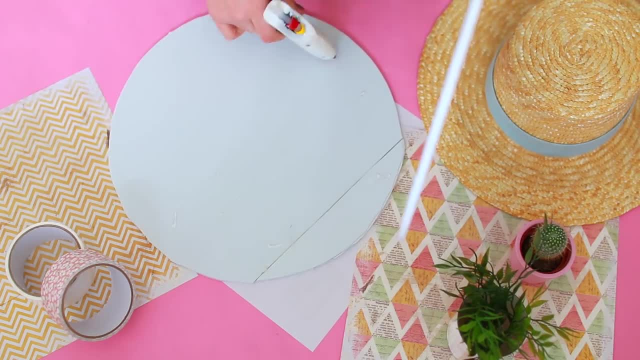 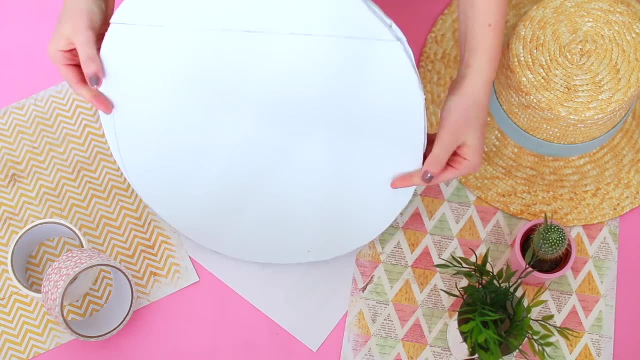 whole fabric and cut them out with your knife of desire. heat up your glue gun and glue both your circles together. and the reason we're doing this is to make a little bit of space for the pins to fit into the board and to make sure the board is thick enough to actually hold your pins. 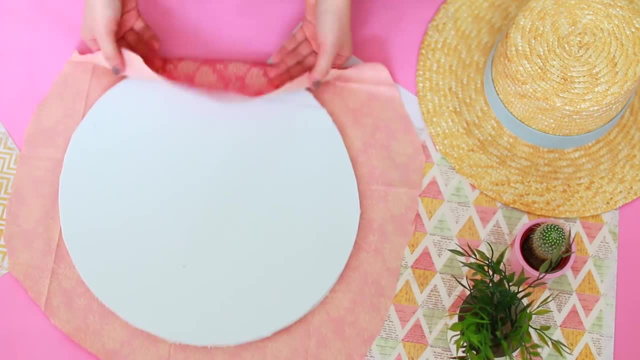 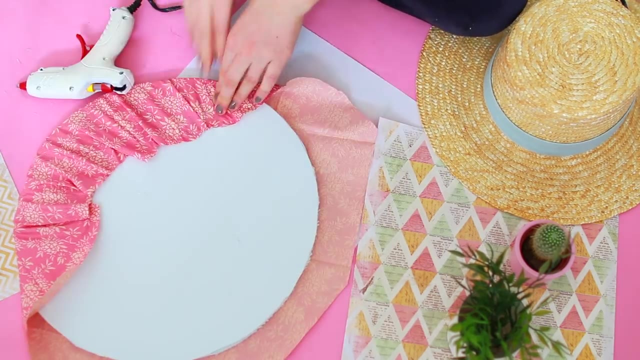 now place your board over the fabric. grab your glue gun and start tightly wrapping the fabric onto the board. now place your board over the fabric, grab your glue gun and start tightly wrapping the fabric onto your board and gluing it in place like so. this should be decently easy.